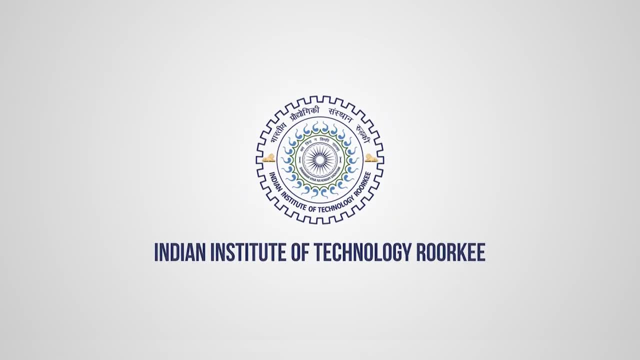 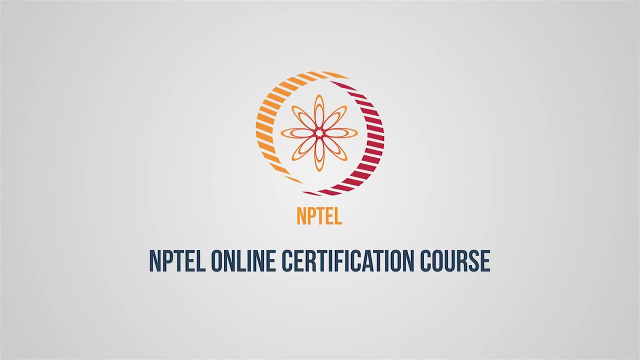 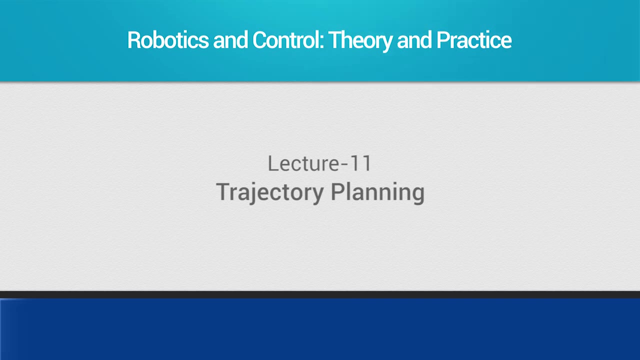 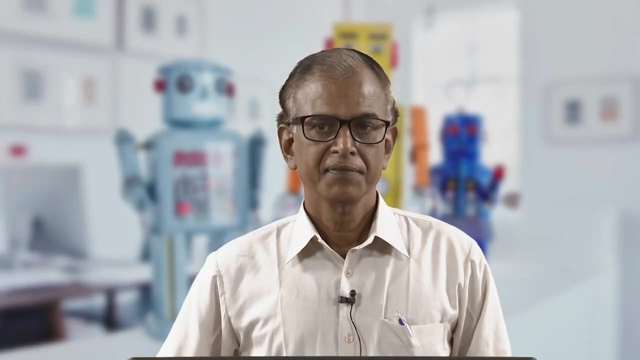 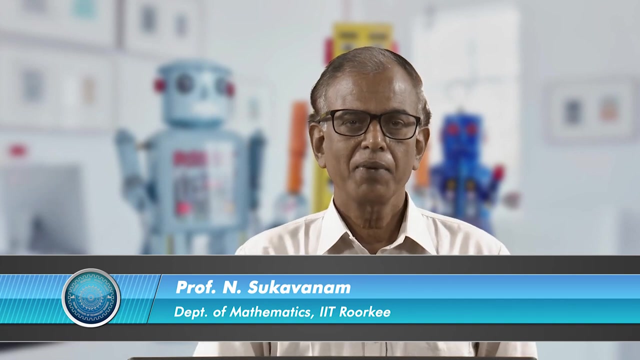 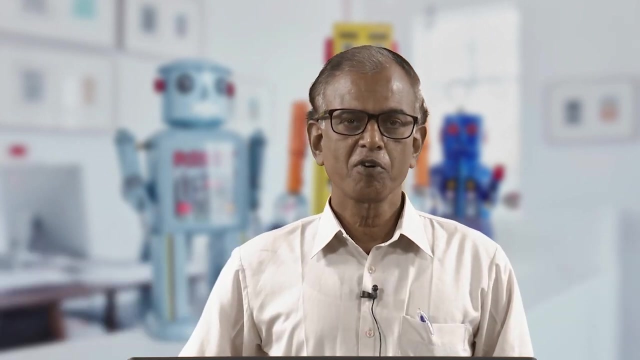 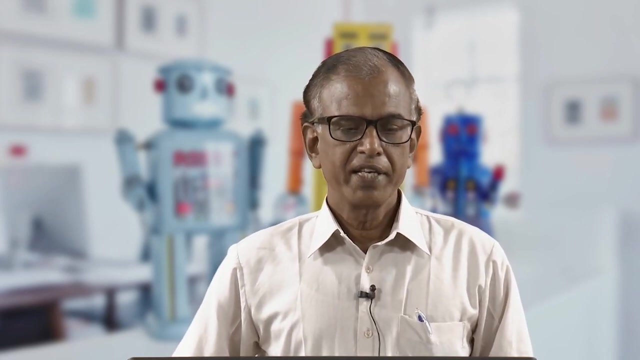 In this lecture we will see how to plan a trajectory for a robot manipulator. So path planning and trajectory planning are very important aspects of a robot manipulator when it is performing a work like pick and place or spot welding, painting or various other tracking problems. So let us see first what is the 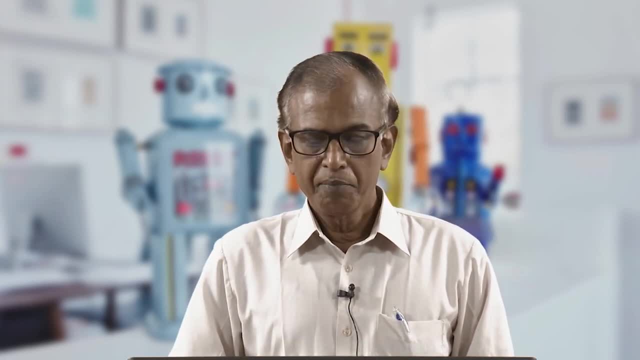 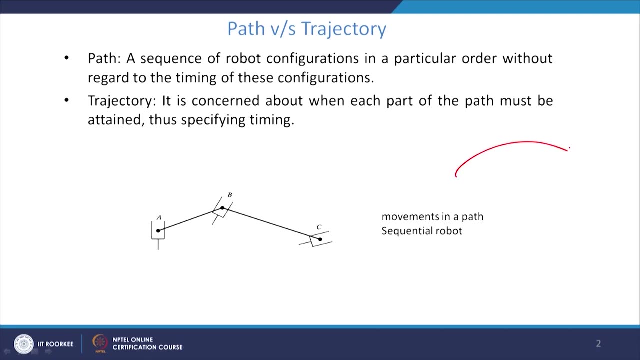 meaning of a trajectory or the difference between a path and trajectory. So a path is a simple curve in the space, where there is no association of the point on the curve and the time. In other words, it is simply a relation between the coordinates. 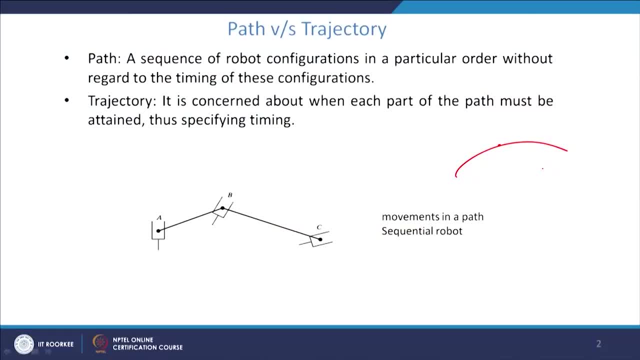 of the point. So, for example, if I write y is equal to x square in the 2 dimensional space, It represent a path only. There is no association of each and every point and the time, but the same curve. if we can give, x is equal to t and y is equal to t square where t is time. 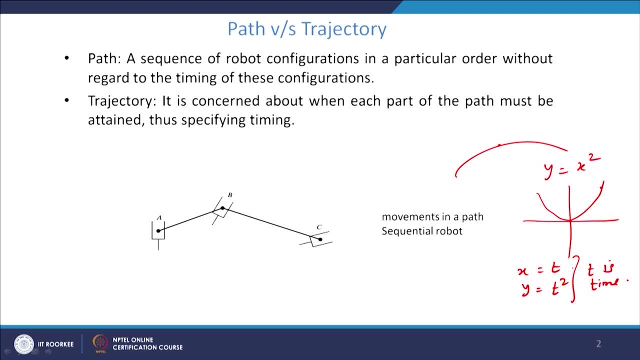 Then it says that the point at time t equal to 0,, the point is at 0, 0., And when t is equal to 1, it is at 1 comma, 1, etcetera. So each and every point on the 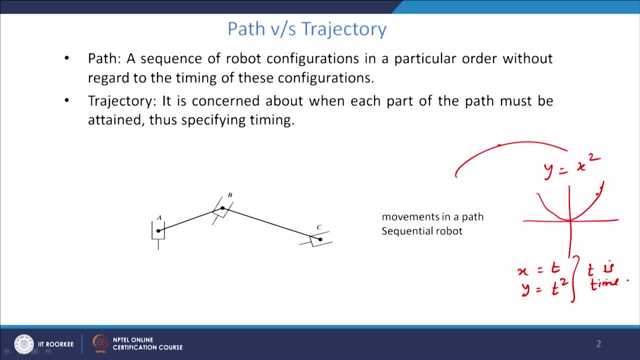 path is associated with a time. So a trajectory is a path to which the time is associated and without association of time, when it when a curve is given, then it is called a path here. So in in robotics the trajectory planning is a very important aspect of a trajectory. 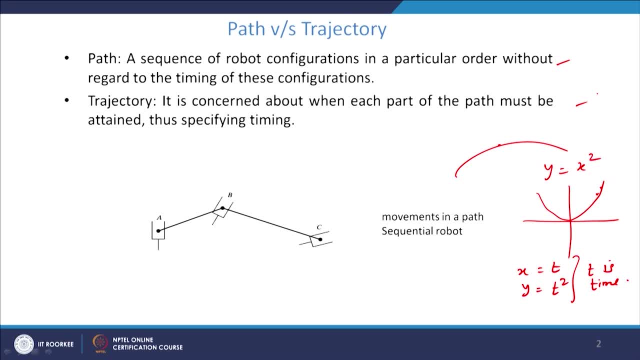 So in in robotics the trajectory planning is a very important aspect of a trajectory. So the end effector. in this picture it is shown that at 3 different time- t 1, t 2, t 3,- the orientation of the end effector should be as shown here, as well as the position is. 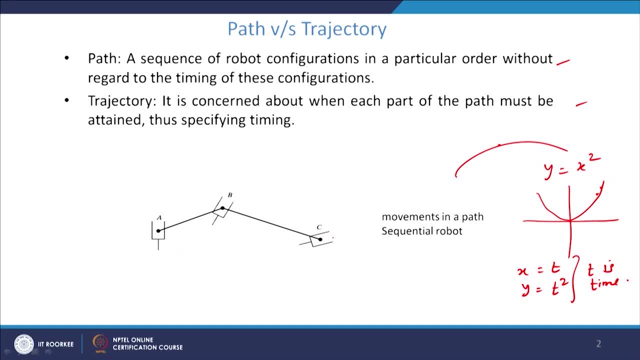 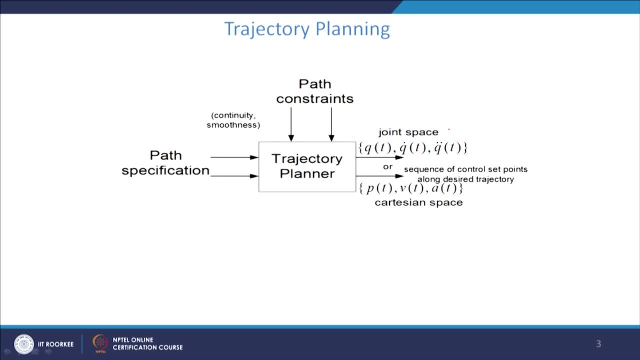 shown as in the picture. So so the trajectory planning is of 2 types for a robot manipulator, That is, joint space trajectory as well as the Cartesian space trajectory. So the meaning of this is, if we have a robot manipulator and if you are interested in moving the manipulator, 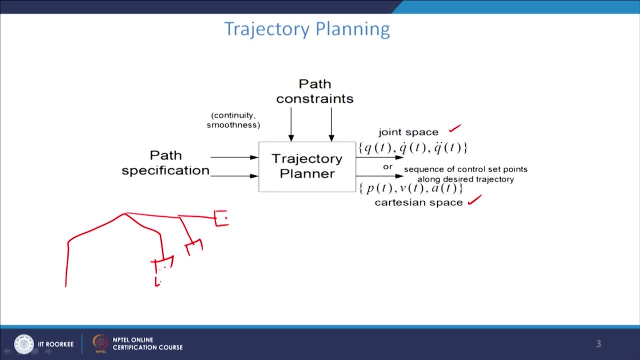 to different configuration like this: So at t equal to t 0, here it is at t 1, at t 2.. So at a 3 different instant of time the robot is having this configuration. So here we. 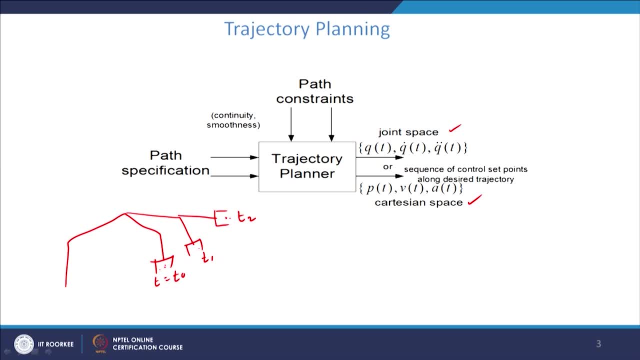 are mainly concerned about the end effector, position and orientation at a different instant of time. So that is called the Cartesian trajectory. It should travel along a path associated with this time. So for performing this Cartesian trajectory, if, if you are giving the angles, that is, q 1,, q 2,, q n, the variables, the joint variables, 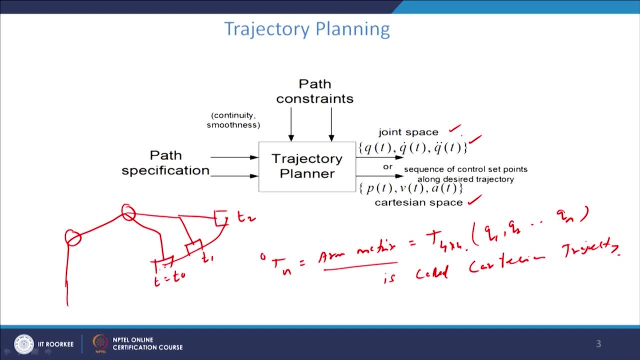 are given as functions of time, then it is called the joint space trajectory. So one can plan to move a robot manipulator either using the end effector trajectory or using the inverse kinematic, But one one if one is given, another is can. 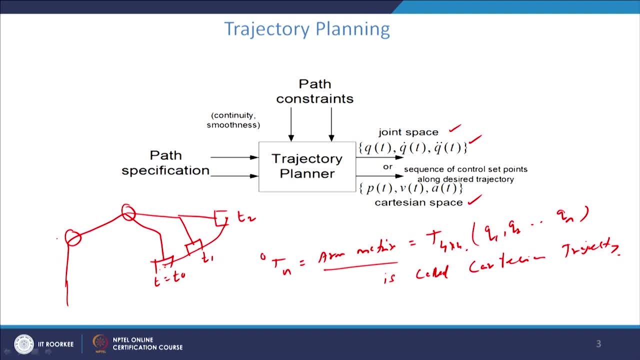 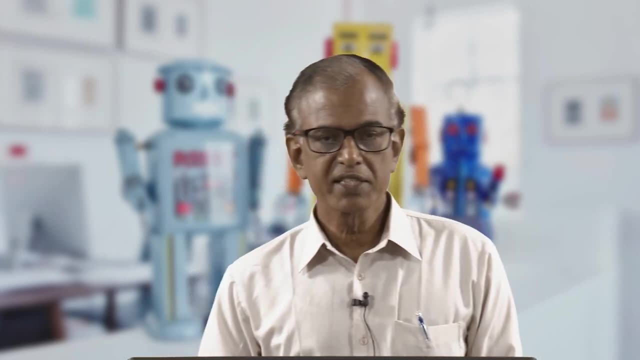 be obtained by the inverse kinematic solution. If the end effector trajectory is given, if the ohm matrix is givenwe know that we can solve the inverse kinematics and obtain the values of q 1, q 2, q n. So if the Cartesian trajectory is given, we can obtain the joint. space trajectory by solving the final, insignificant metabolic situation, Punkt I. hey, I am done. indeed it is in hilarious resolution. So we nothing done, but it is done. so we are achieving the chase problem, If the robić. 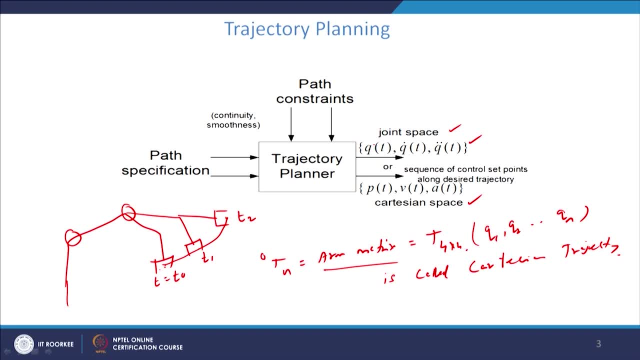 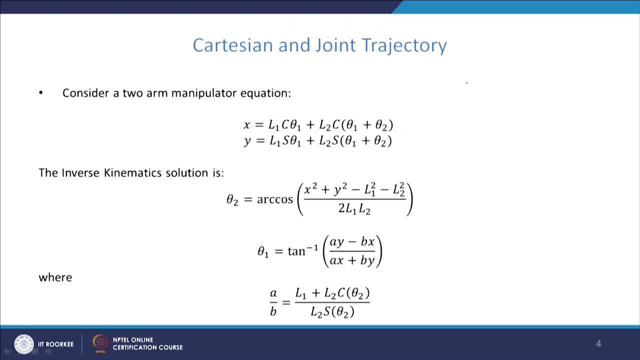 solving the inverse kinematics. Similarly, if the joint trajectory is given directly, by substituting in the kinematics equation we can get to the end effect trajectory. So both of them are related concepts. So here for examplefor the two arm manipulator. 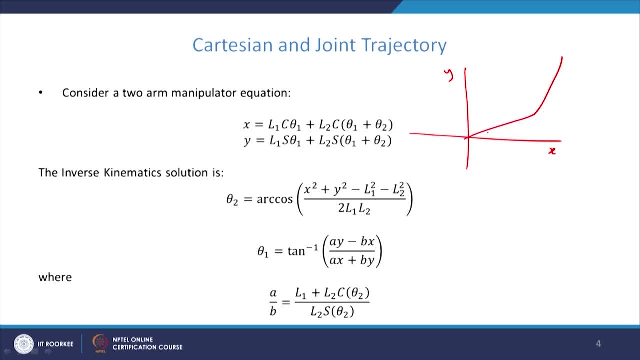 x- y axis. we have a manipulator like this and the actuators at this joints. the angle is measured at the x axis, theta 1, and this is theta 2. the end effector position is x- y. So x is given as L 1 cos theta 1 plus L 2, cos theta 1 plus theta 2, where L 1 is the. 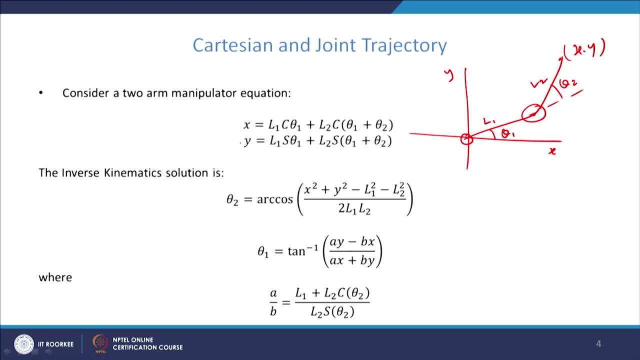 link length and L 2 is the second link length. So this is a verysimple geometrical concept. we can easily obtain the. So from here we can solve theta 1 and theta 2 byusing simple algebraic manipulations. and this a and b are: 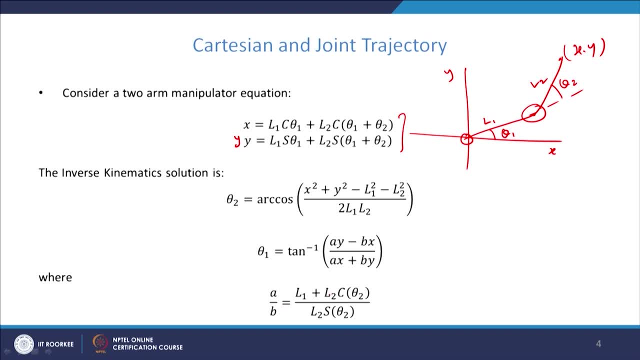 given by this expression as a equal to L 1 plus L 2 cos theta 2, and b is L 2 sin theta 2, and by substituting we will get the values of this thing. So, given the equation for x and y, we can obtain the inverse kinematic solution, theta. 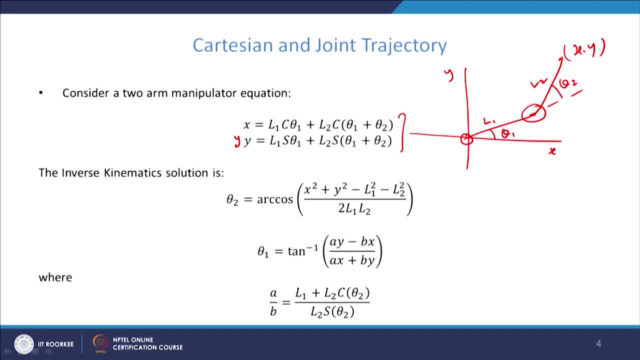 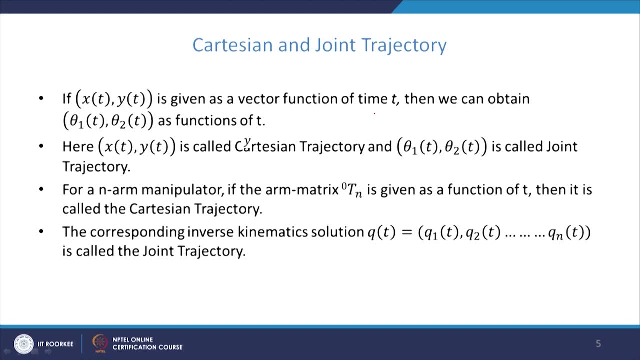 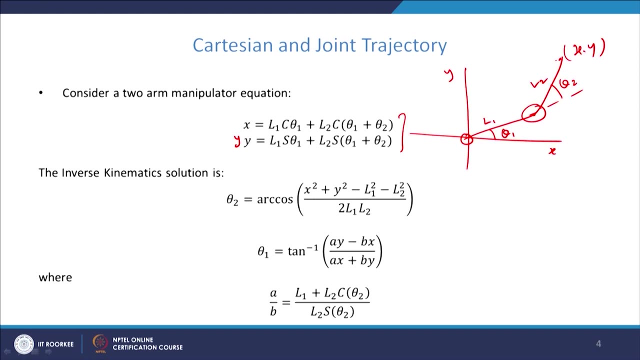 1 and theta 2 in this manner. So now, if we plan a trajectory, if x of t, y of t is given as a function of time, thenwe call it as the Cartesian trajectory, that is, That is, if you want that the end effector should travel along a straight line, should. 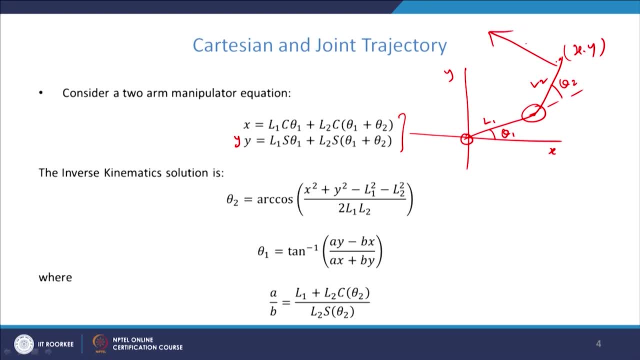 travel along some straight line in this manner, then the equation of this straight line can be given as a function of time. at each and every instant, what should be the position of the end effector? So that can be calculated. So for each and every end effector position we can solve the inverse kinematic. 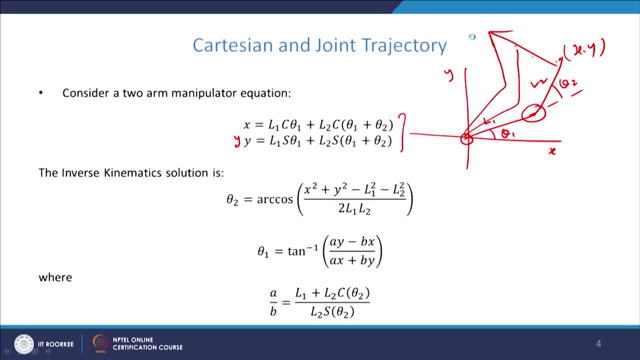 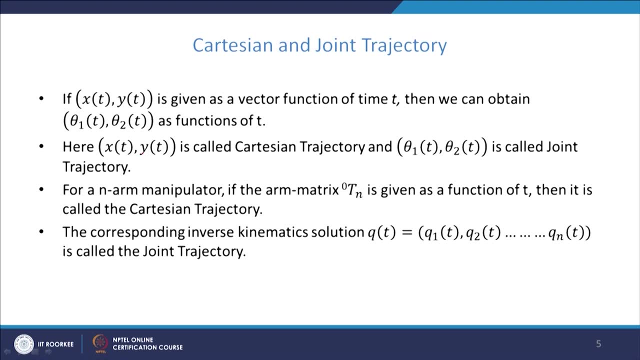 So if the end effector position is given as a function of time, that is the Cartesian trajectory. and if you solve the inverse kinematic and obtain theta 1 and theta 2, that is the joint trajectory for this thing, the 2 ohm robot manipulator. 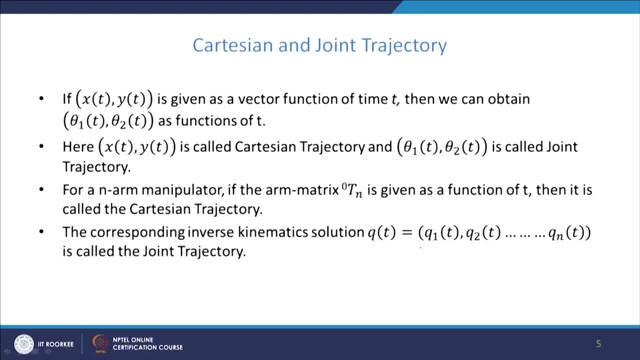 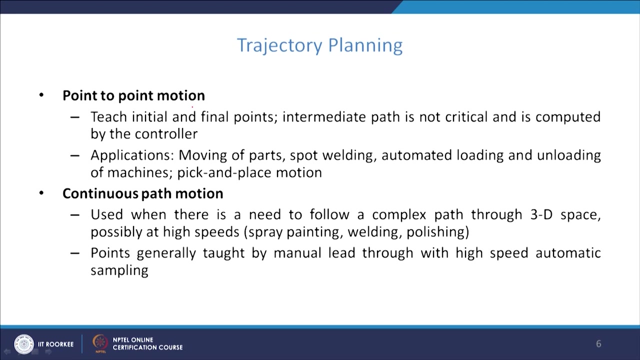 So in general, for the n, n ohm manipulator, if the 0, T, n is given as function of time, it is called the Cartesian trajectory, and the angles are given as function of time, it is called the joint trajectory. Now the trajectory planning is of two types: point to point motion, as shown here. 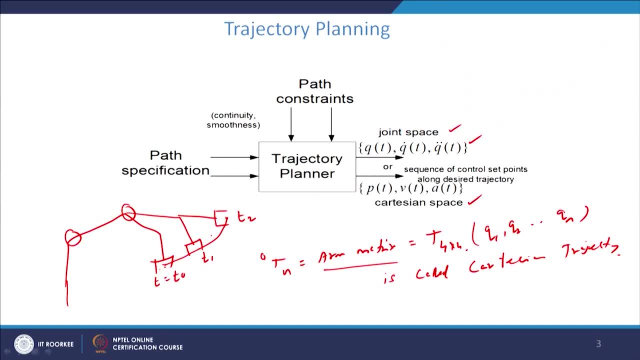 So at different instant of time the positions are given. So in this point to point motion, we are not concerned about the intermediate position. that can be calculated by using some simple formulae, Because we are not specific about the intermediate position of the end effector. only aim is to 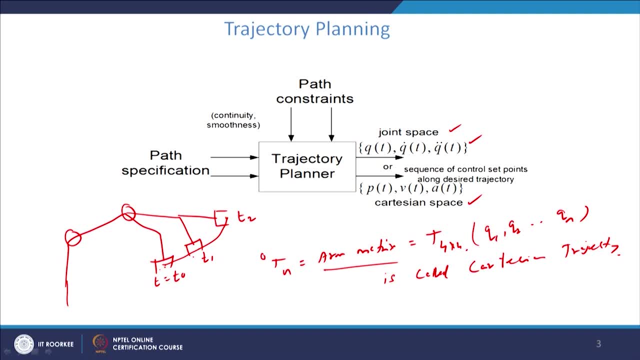 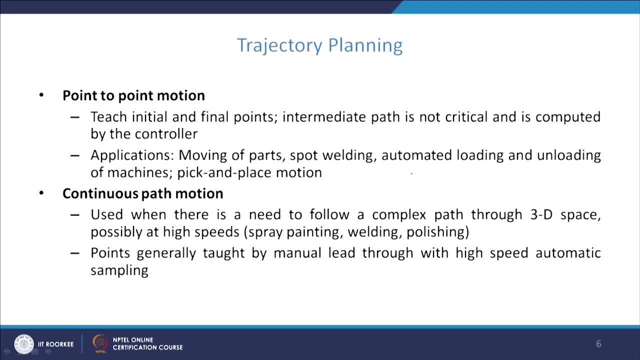 reach these three specific points at this three instant of time which can be planned. So that is point to point motion. Like, for example, the loading and unloading work or the spot welding type of things can be done using the point to point motion. 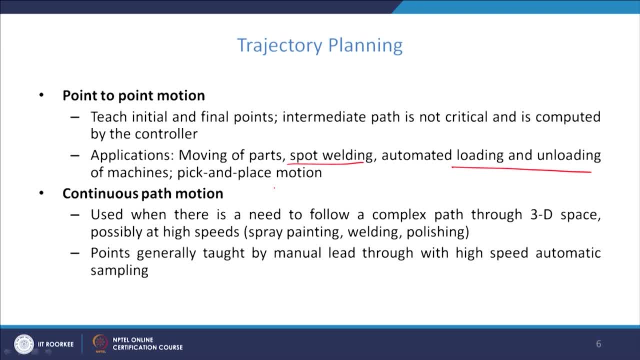 Because taking an object and putting it, only two positions and orientations are important and the initial and final time are important. Intermediate positions one can calculate, Calculate by various types of form, But continuous path motion is. we are not only interested in the initial and final, but all. 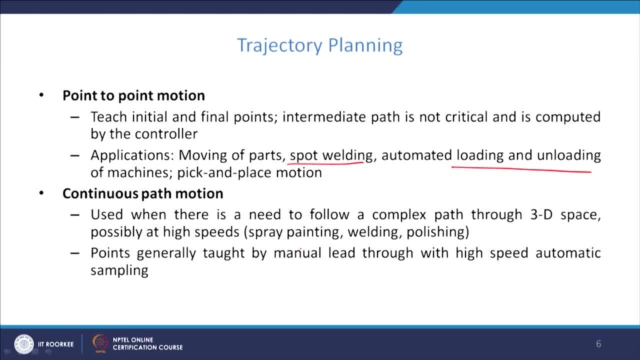 the intermediate positions are also important. they are also to be planned in a suitable manner. So, for example, the spray painting welding, continuous welding of metals, etcetera. So they need a continuous travel of the material. So they need continuous travel of the material. 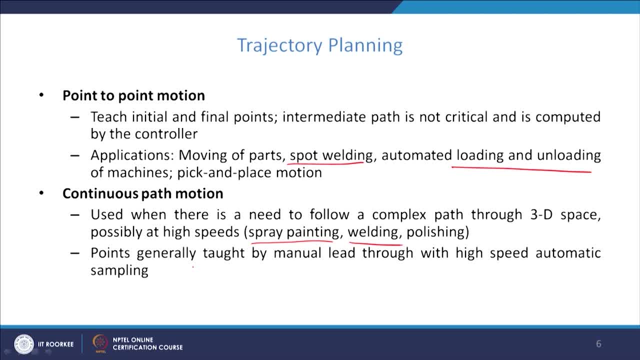 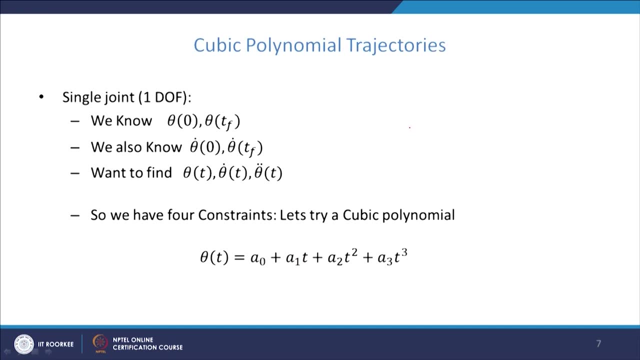 So they need continuous travel of the material end effector, of a robot manipulator. So in both the cases we can follow the procedure of finding the trajectory using polynomials. So generally initial position and final positions are given, or more conditions may be given. So if we know the at the zeroth initial time. 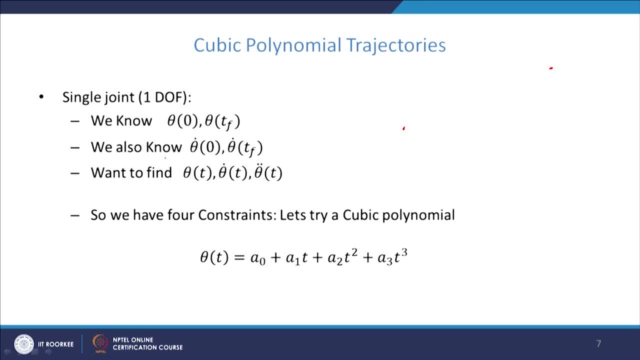 t equal to 0 and the final time t f. So the position 0, theta of 0 and theta of t f is known and the velocity at initial time and final time, the derivative theta dot, is known. Then we can find the intermediate values of theta of t for various values of t. So how? 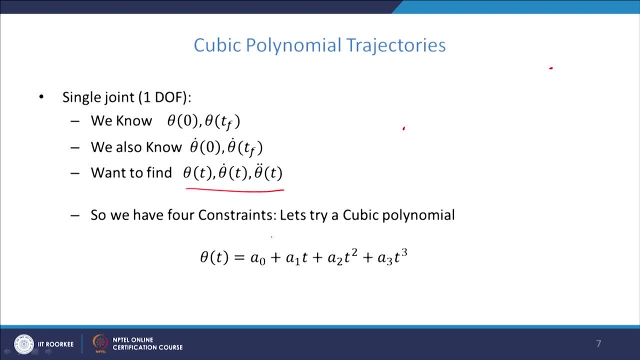 to find that can be easily fit here. So because there are four conditions, given theta 0, theta t f and derivatives at the two points, So we can consider a polynomial of degree 3, then by substituting the values, we can obtain the coefficients a 0, a 1, a 2, a 3.. So it is a very standard way of fitting. 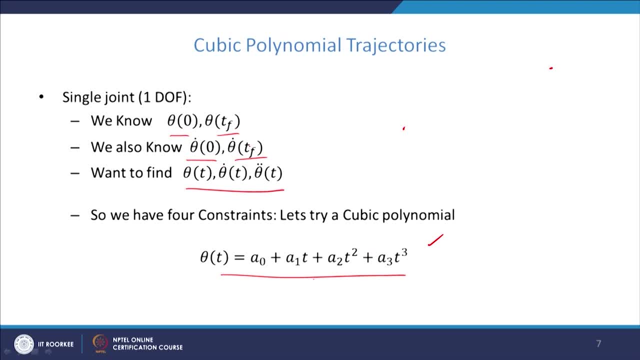 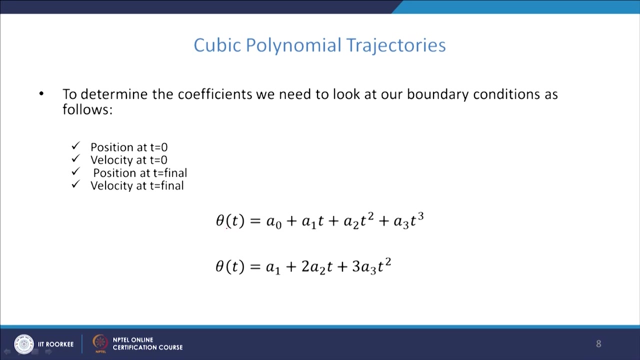 a polynomial for given constraints. If there are n conditions given, like this, then we can fit a polynomial of degree n minus 1. So that there are n minus n coefficients and which can be obtained uniquely by solving. So we can easily see that if theta of t is this one, its derivative theta dot of t is: 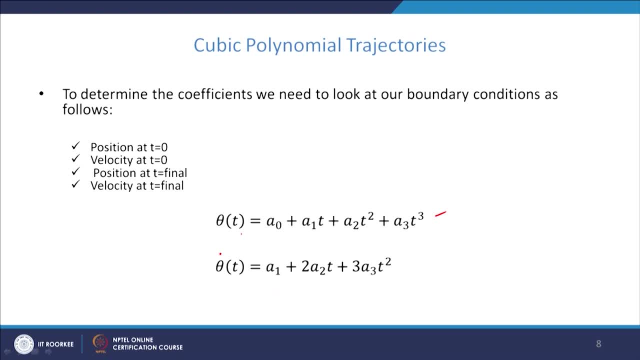 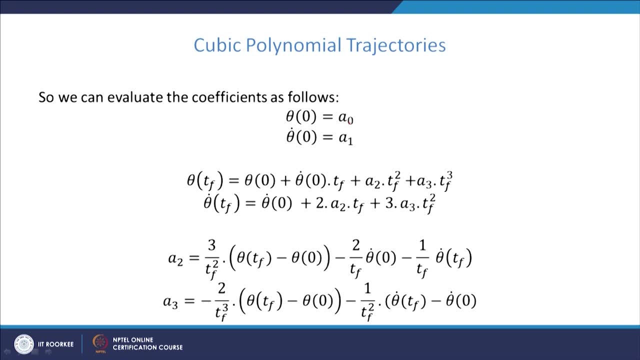 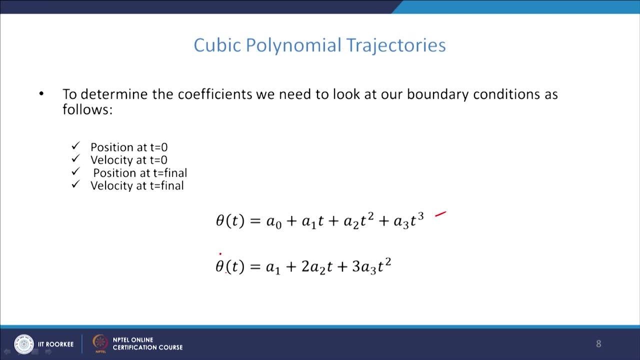 given. by this directly differentiating And then substituting t equal to 0, we will get theta of 0 is a 0 and the derivative. if you put t equal to 0, we get a 1, a 1 is theta dot of 0. So these 2, so these 2 are. 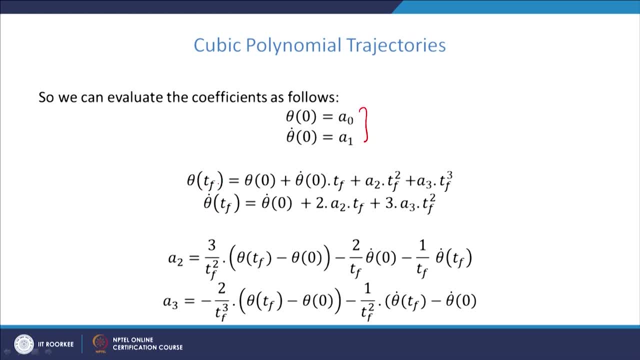 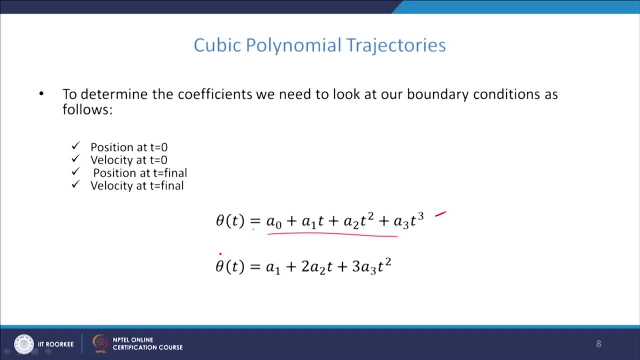 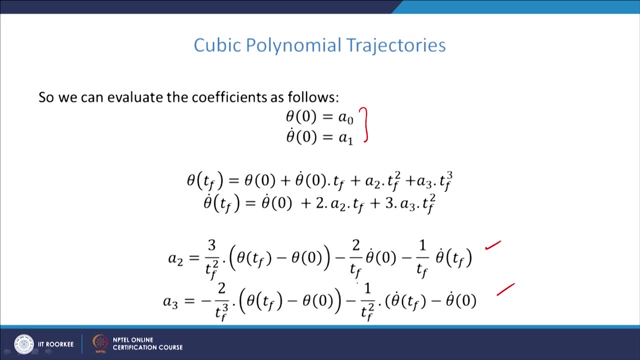 directly obtained. Now, by substituting the final time t f in this expression, t f in this expression, we get Already. we have obtained A 0 and A 1. So A 2 and A 3 are obtained by this simple procedure. 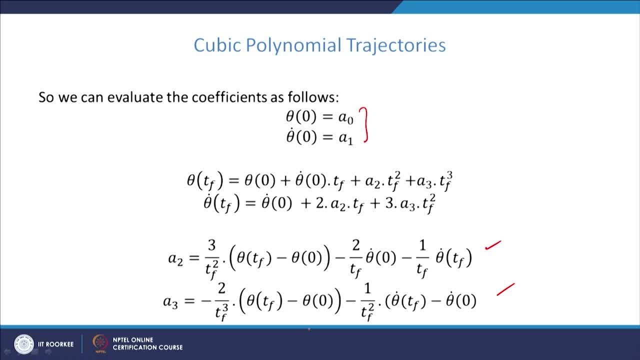 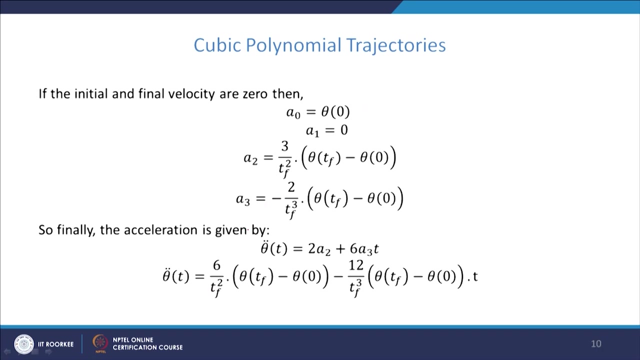 by solving the two equations. So by this procedure we are able to get, given the initial and final condition and initial and final velocity, we can fit a curve theta of t for all the intermediate positions. So this procedure can be adopted for any number of such conditions. 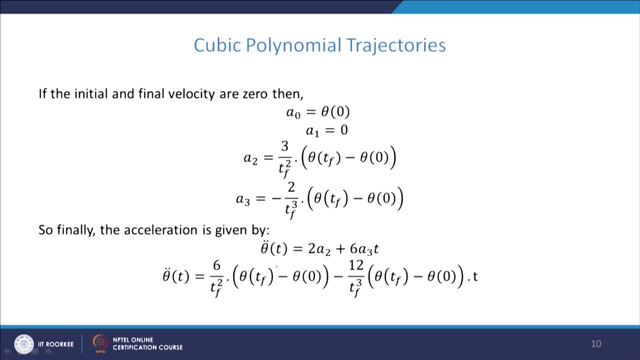 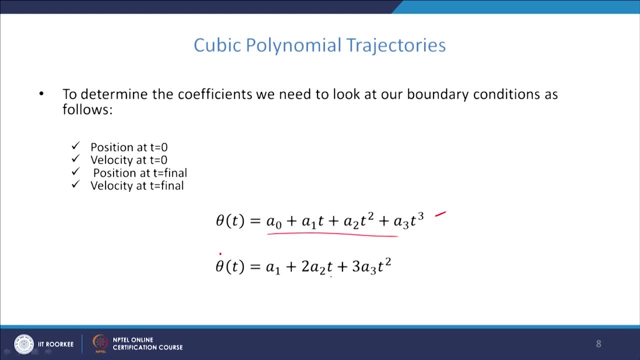 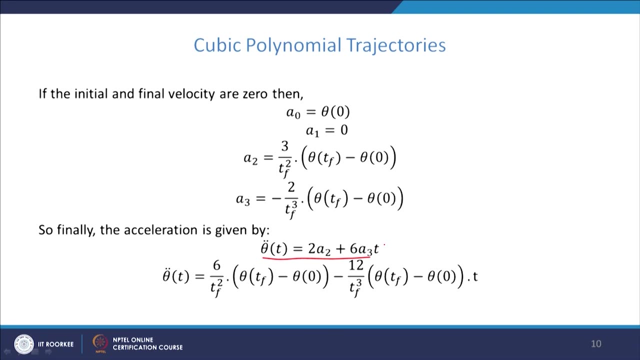 Now, if we consider the second derivative of the theta with this polynomial first derivative, is this: further, if you differentiate, we will get 2 A 2 plus 6 A 2 t, this expression. And now if you substitute A 2 and A 3 value, we get this acceleration. the second derivative is called the acceleration. 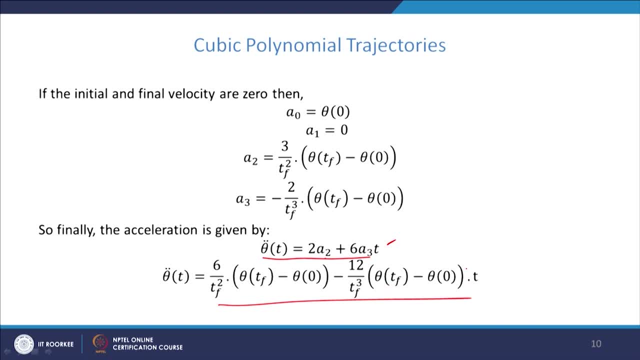 is given by this expression. Now we can observe that when we put t equal to 0, this acceleration is constant. some value is obtained. So it is little bit of disadvantage when a robot is moving at t equal to 0. So the acceleration is some nonzero value. it means there will be a sudden discontinuity. 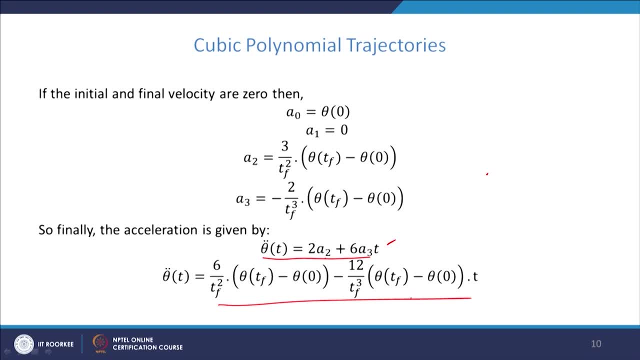 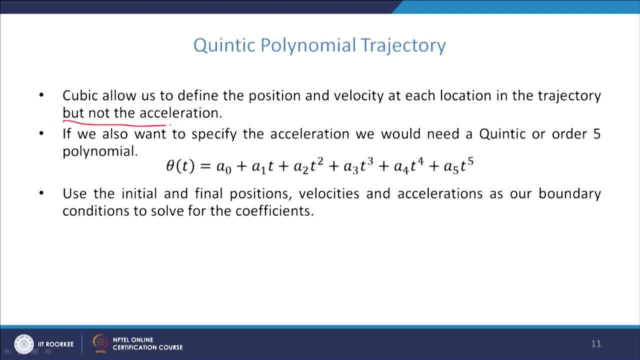 in the acceleration at the initial time. So here for a smooth motion of a robot manipulator. if there is a discontinuity at the in the acceleration, it is not desirable. So here we see that we cannot specify the acceleration on our own, Because automatically we have. 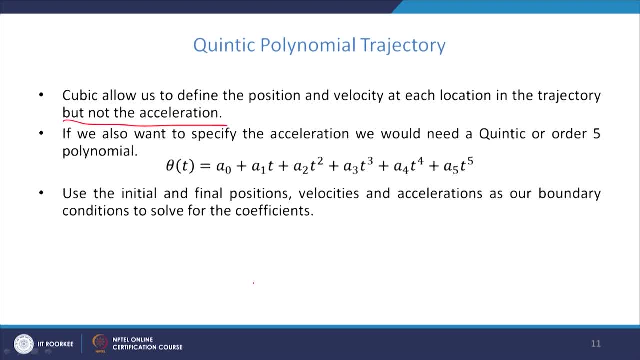 it takes some value at t equal to 0. So to avoid that we can increase the number of polynomial, the degree of polynomial. So if we have initial position, velocity and acceleration is specified, and similarly final position, velocity and acceleration is specified. So there are 6. 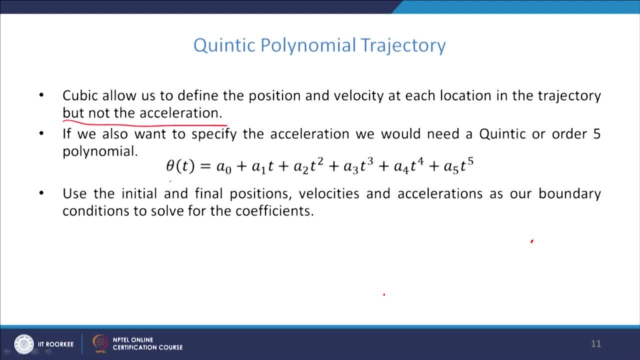 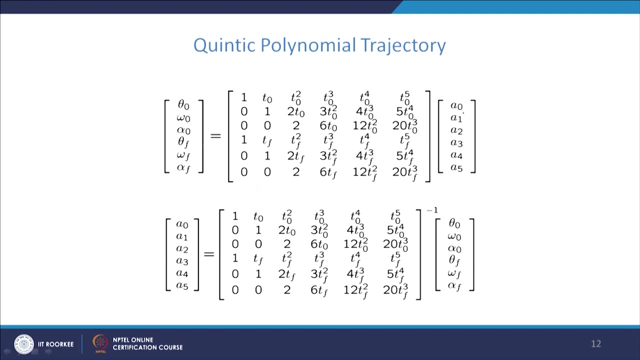 conditions. Using 6 condition we can fit a polynomial of degree 5 like this, and then, using those 6 condition, we can find the constants a 0, a 1 up to a 5 in a very simple manner: directly substituting. we get a system of equation and the coefficients can be obtained like: 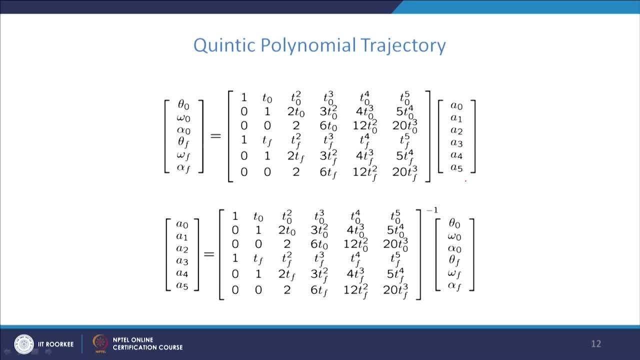 this: a, 0, a, 1, a, 2 up to a 5.. Is obtained by the inverse of this matrix multiplied by the known values. This is the. it is given that initial position, initial velocity, initial acceleration- This is final position, final velocity, final acceleration. So if this 6 values are given, we can substitute: 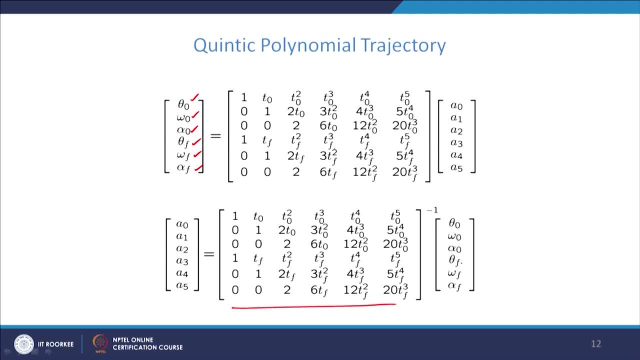 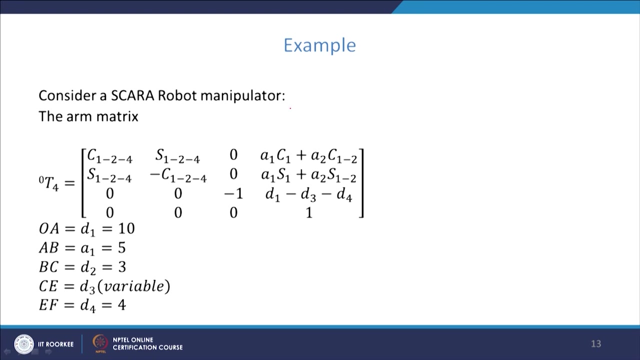 and then multiply by the inverse of this matrix, we obtain the coefficient directly, like this. So it It gives the fitting of a polynomial. if some constraints are given for any type of problem, So this can be applied for the robot manipulator problem like this. So let us consider a, the 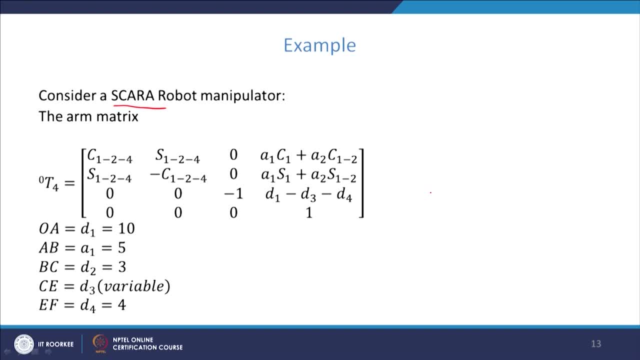 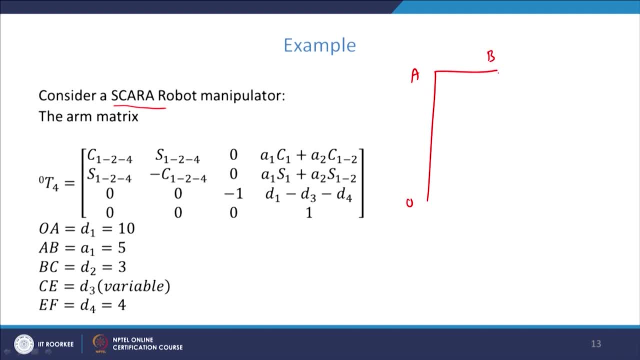 is H. Now let us take the frequency a and B, And here there is a revolute joint and this is prismatic joint. So the first joint is a revolute one and the second is also revolute. the third one is a barrel- После pereir attacks for widow. So we simply make these guys. 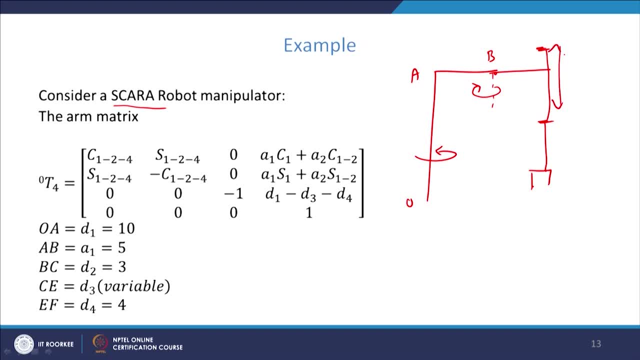 study as Manual Holler Filter. A sample of this machine can be pleasant as a formula for the action analysis. So let you get the detail of this gamut frog спасi colocar. hydrogelgest Largan is a prismatic moving above and below, and the fourth one is a revolute joint. So we 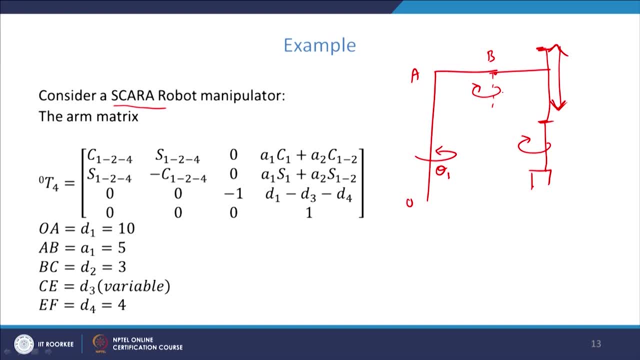 call it as theta 1, this rotation theta 2 and this is theta 4, and O A, B, C, D, E, F. So if we take O A to be 10, this length, and A B is 5 here and B C is 10.. 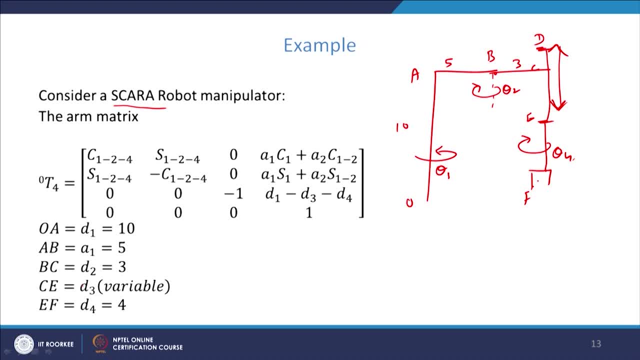 So this 3 C E, it is a variable, this one from, because it is going up and down. the C E is a variable and E F is 4, E F, the value is 4 here. So the using the D H algorithm. 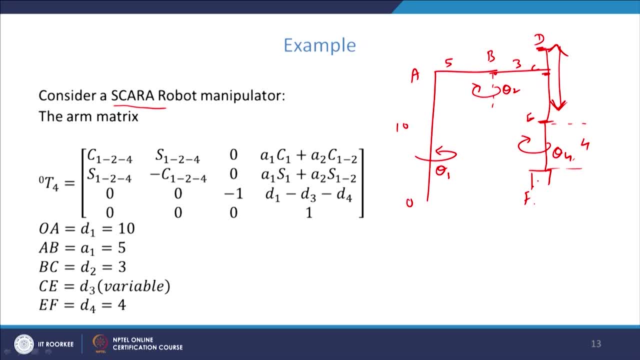 and then fixing all the coordinate frames and then writing the parameters of the manipulator, we can easily calculate the arm matrix 0, T, 4 to be like this: The relation between the base frame, x, 0, y, 0, z, 0, the end of vector frame here is: 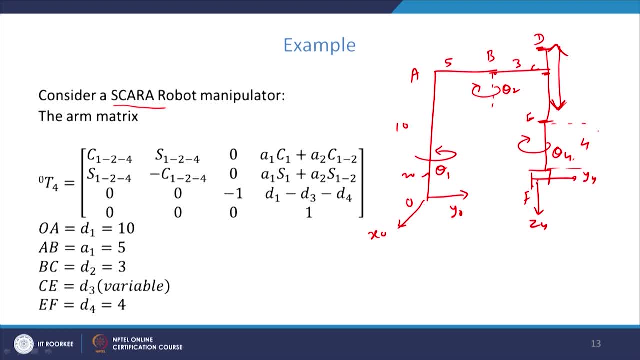 z, 4 y, 4 x, 4.. So the relation between the end of vector frame with respect to the base frame is given by the arm matrix like this for the given parameters. Now, if you want that the robot should travel between 2 points, that is 2 instant of time. 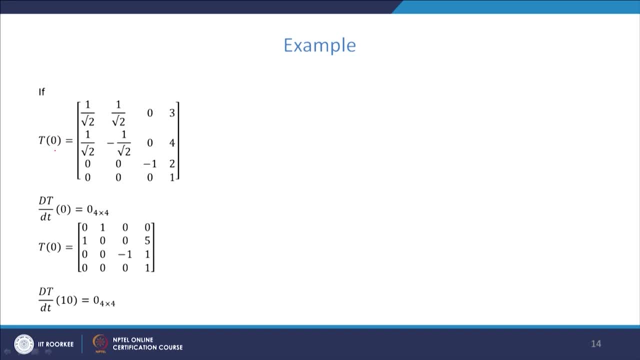 if you are giving at t 0, the time t equal to 0, t of 0 is given by this expression and this is 10.. Ok, T at time instant 10 is given by the homogeneous transformation as given here. So it means: 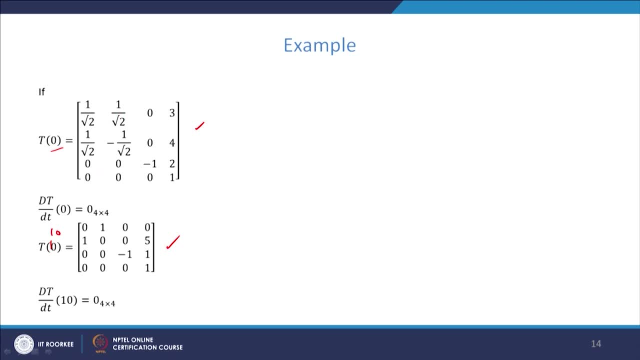 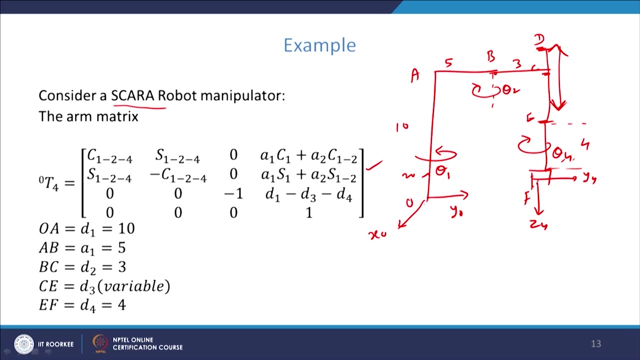 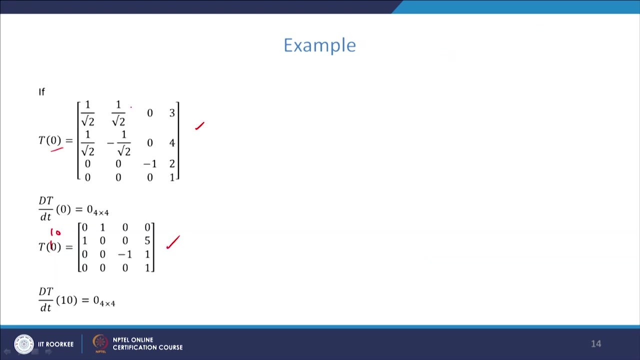 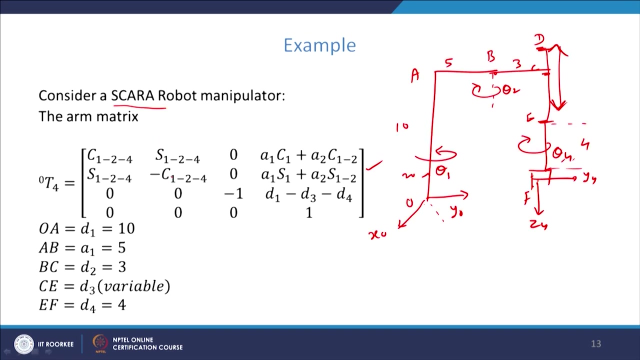 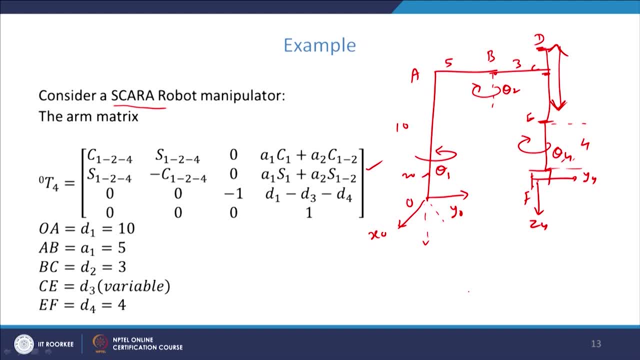 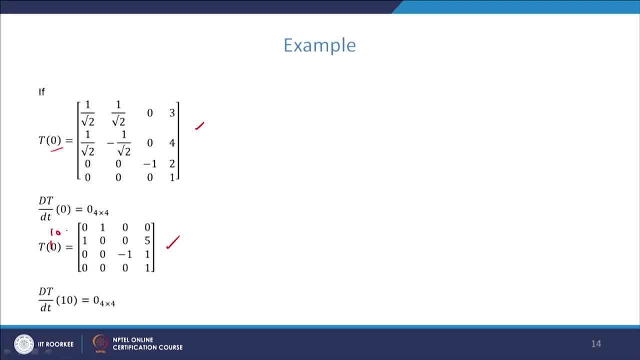 z coordinate of the end of vector. So it is 0, 0 minus 1.. So as so as given here. Similarly, at the time t equal to 10 units, the x axis will be 0, 1 0 of the end of vector. 0 1 0 is. 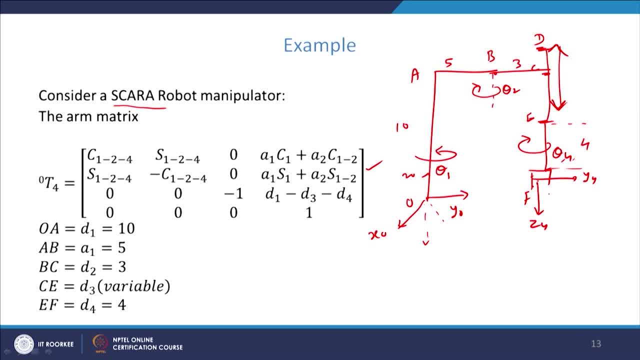 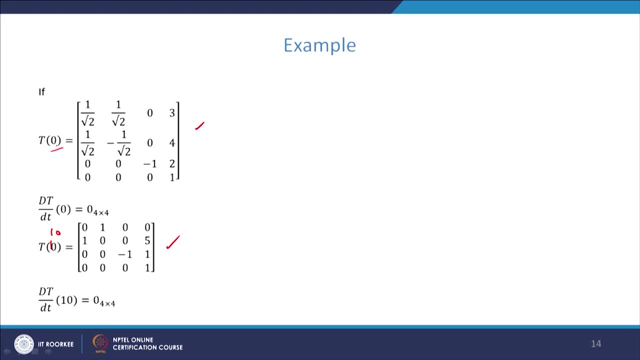 the y axis here for the base. So the x axis of the end of vector will be parallel to the y axis of the base at t equal to 10.. So it should turn so much of angle so that it adjust itself from time t equal to 0 to this one, And the origin of the end of vector is 0, 3. 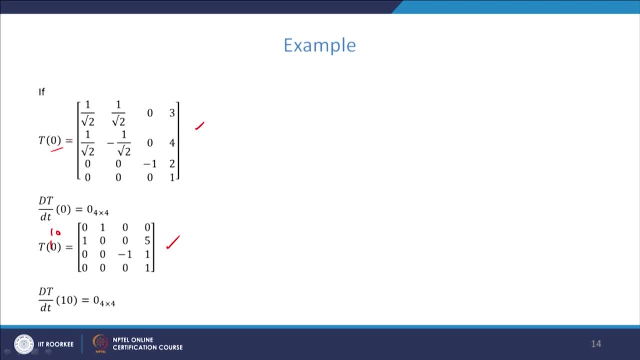 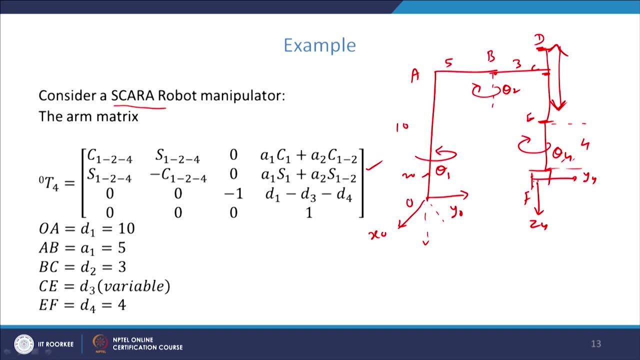 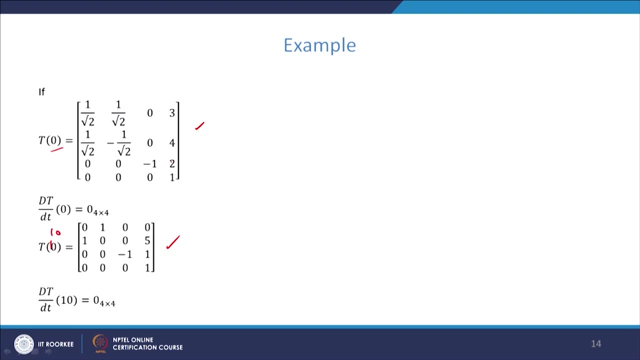 0, sorry, 3, 4, 2 at time t equal to 0, and it is 0, 5, 1 at time t equal to 10.. So it it is shifting. the origin should be shifting to the values as given here. the fourth column. 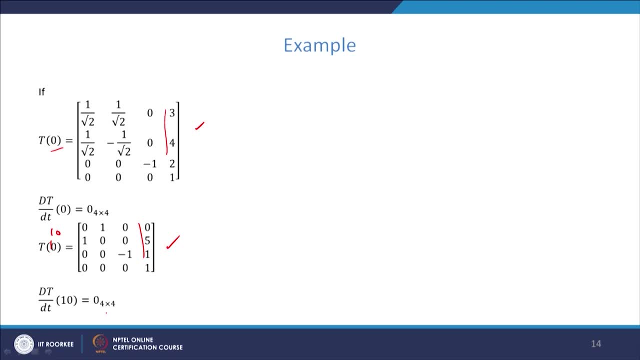 of the this thing. So for performing this position and orientation between this two time instant, 0 and 10.. Similarly, the velocity of the end of vector is 0 at t equal to 0 and it should stop at the t equal to 10.. So what we have is we have 4 conditions at 2 instant of time. So 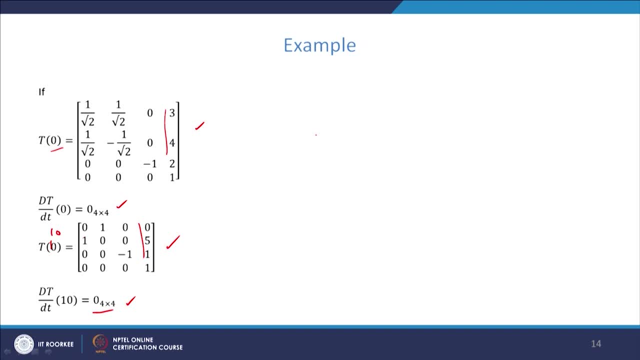 we can simply fit a third degree polynomial with 4 coefficients. So we will write that the end of vector 0, t 4, as a function of t equal to 0. So this level of dessa del t is little bit I, not a little bit outside. 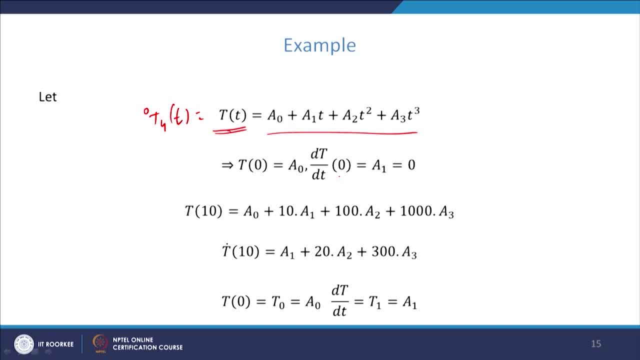 So this is responsibility and which are really can be calculated from. look at these three points which are 0 for from this way into here to 0 in this way. So t isQuery 1, the Truth limit, stepping out, it will be d t at t 1T of t 1, because t of 0 it is special one. 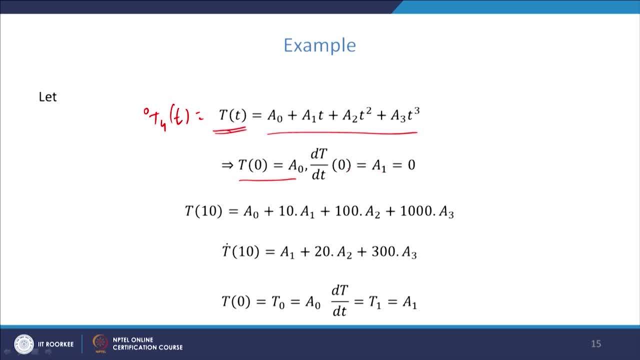 So t is demonstrations of time should follow this polynomial trajectoryT equal to 0. it is the A 0 can be calculated directly to be t of 0. so A 0 is the matrix given by t of 0, as given here, And when we differentiate it we will get A 1 is nothing but d by d t at. 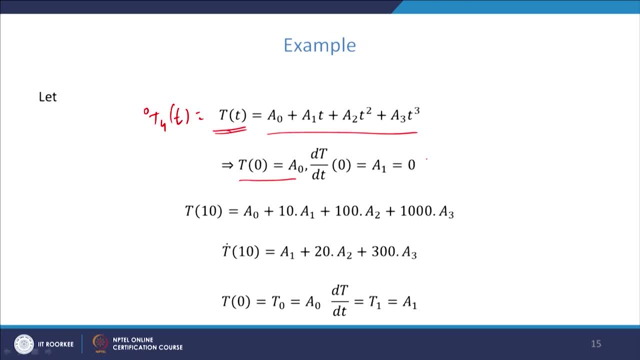 0, that is equal to 0 here here. So A 1 is the 0 matrix. Similarly we can find: when we substitute at t equal to 10, small t equal to 10 in this expression we get this value that is equal to as given. 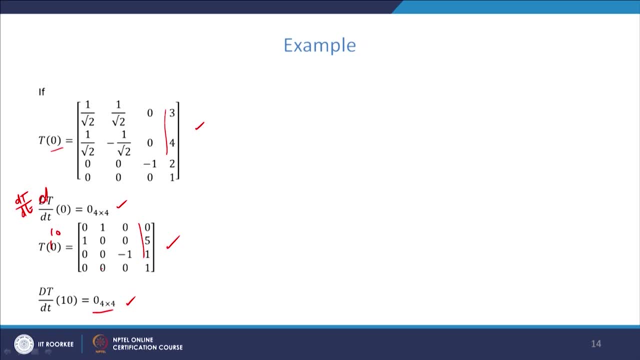 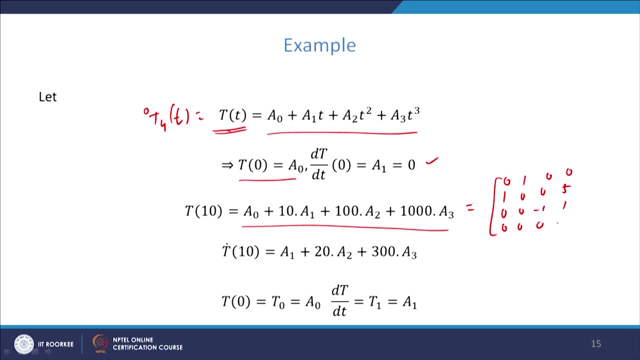 by this one: 0, 1, 0, etcetera. So we get t of 10, as given here, and the derivative is 0. Now, when we solve these two equation, we will get the values of A 0 and A 1.. 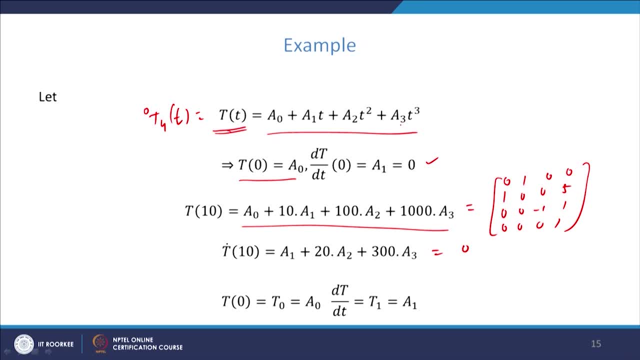 So A 0, A 1, A 2, A 3, etcetera. So once we obtain all these four coefficient matrices by substituting we get the entire trajectory. So the trajectory planning is performed in this particular manner for the given SCARA robot manipulator. So the procedure is same. 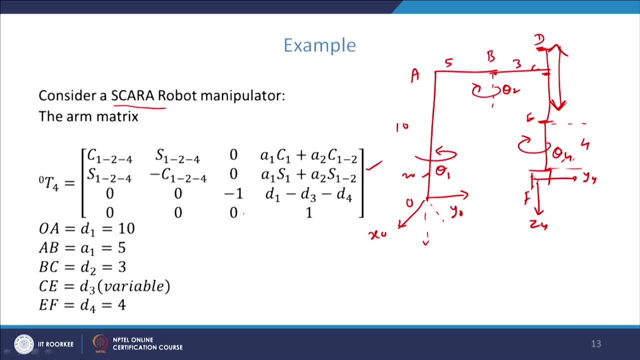 for any type of manipulator, once the initial final conditions are given, whether it they are. So if there are two conditions, we will fit a polynomial of degree 1, and if there are n conditions, we will fit a polynomial of degree n minus 1 and find a trajectory. So 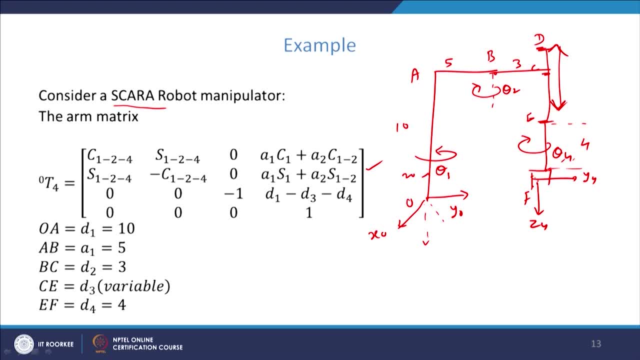 that one can find the end effector position for each instant of time. Whatever we have done here, it is the Cartesian trajectory because it is giving the end effector position as a function of time. Now, if you saw all the inverse kinematic solution for each and every instant of time. 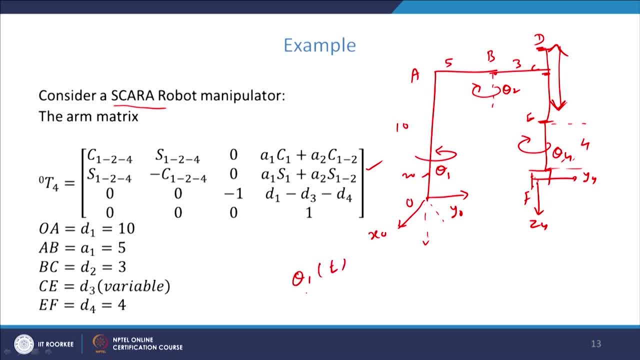 we will get theta 1 and theta 2 as a function of time, d 3 and theta 4 by solving inverse kinematics. So this is called the joint trajectory. So Iторов did nothing else so far either. right lie Bolzano. 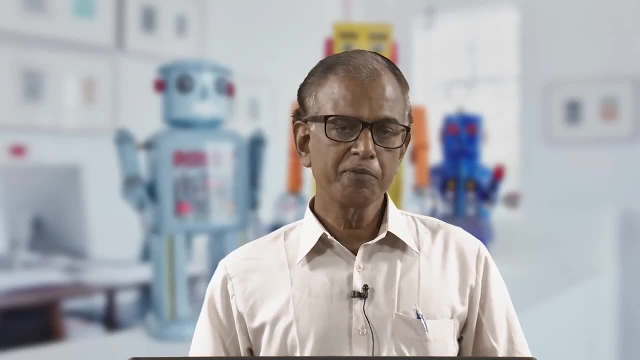 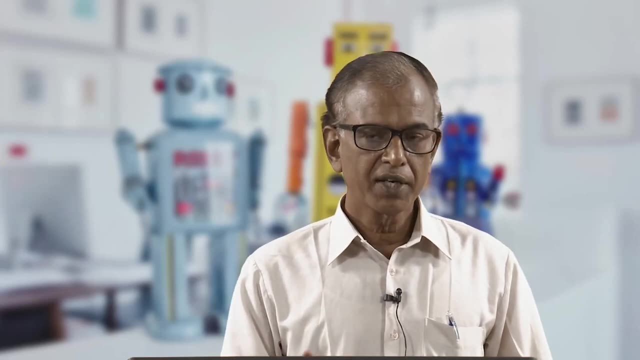 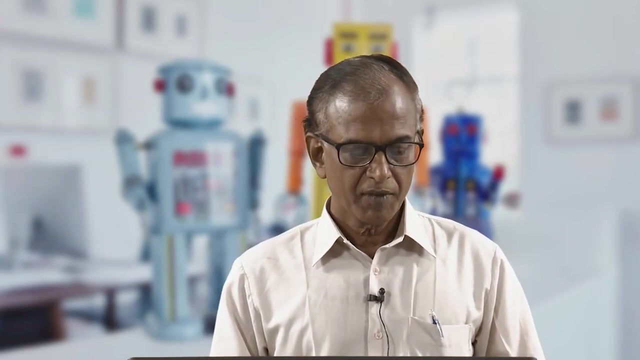 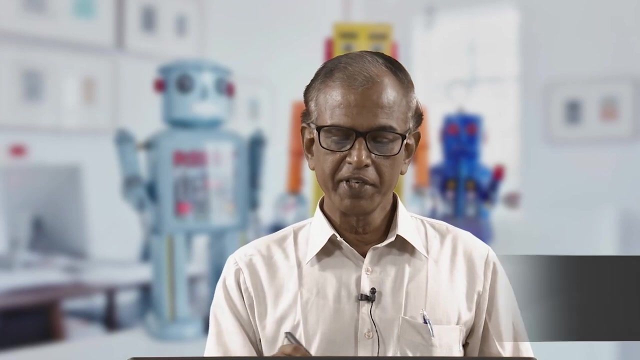 seinee 1 and 1.. For any type of robot manipulator we can calculate the Cartesian trajectory or the joint trajectory by using the number of conditions. If there are n conditions, given initial and final conditions, then we can get, we can fit a polynomial of degree n minus 1 for the Cartesian trajectory. 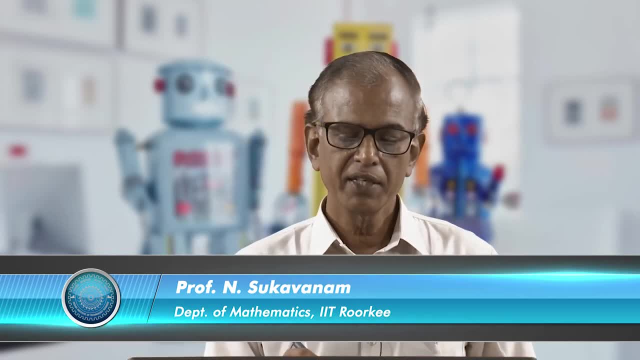 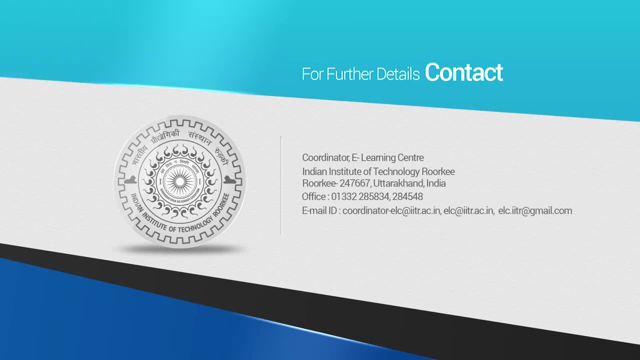 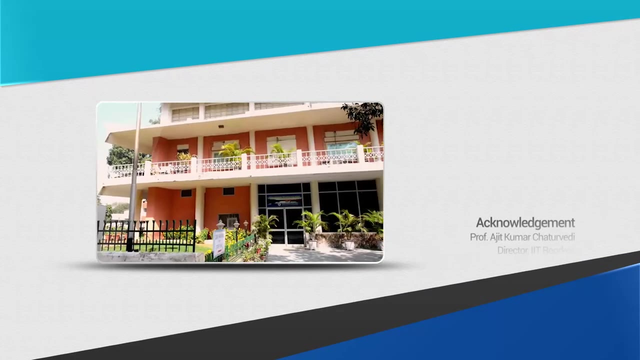 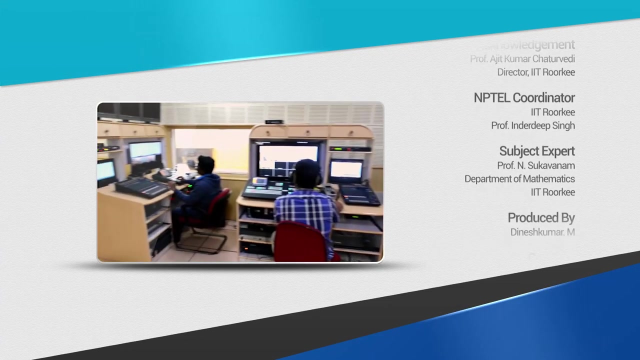 and then solving the inverse kinematic solution, we will get the joint trajectory of the manipulator. ok, Thank you.